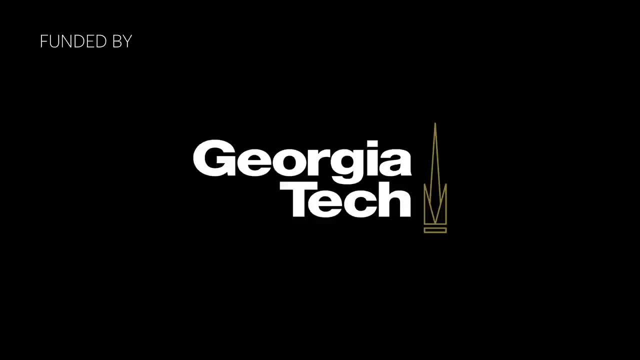 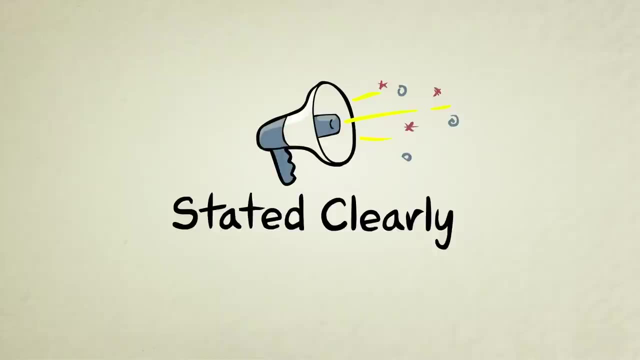 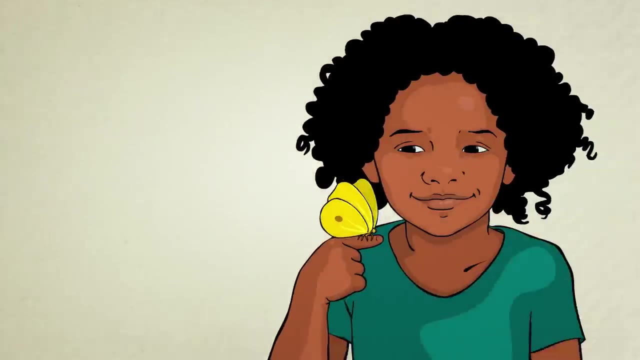 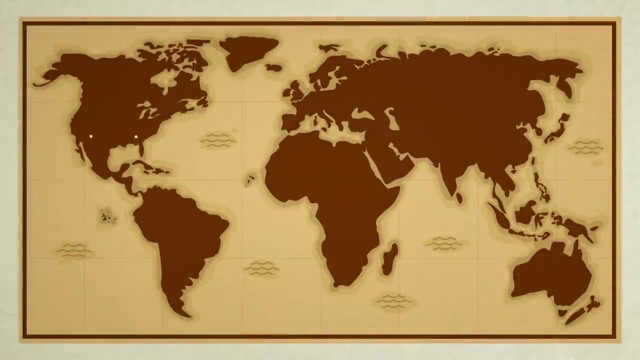 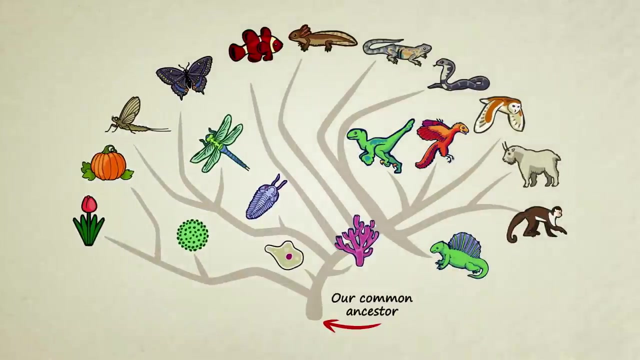 A full scientific explanation for the origin of life does not currently exist, but research groups around the globe are tackling the mystery. Here we'll take a look at a few of their discoveries. Darwin's theory of biological evolution tells us that all life on Earth may have originated. 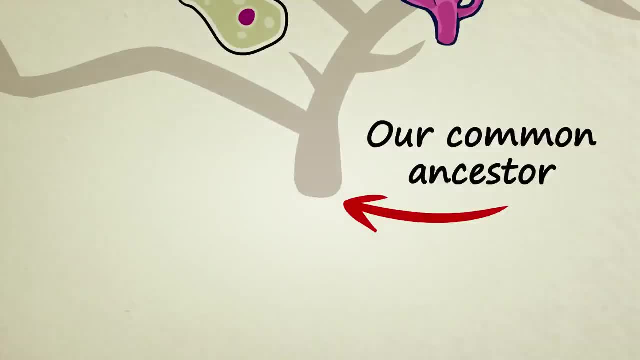 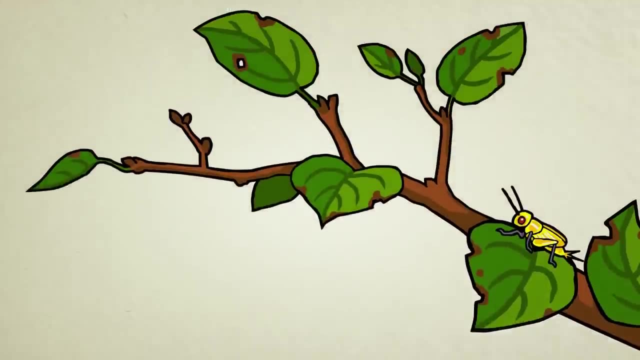 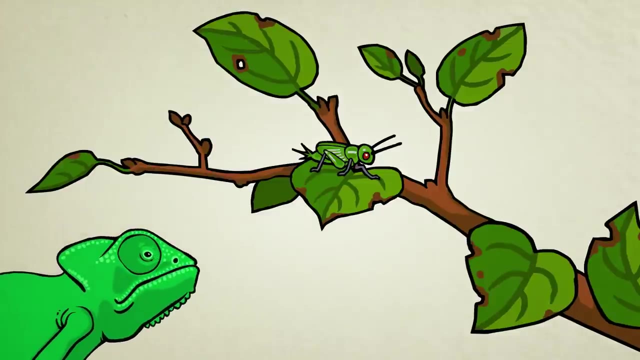 from a single, relatively simple reproducing creature living in the distant past. This idea is based on many observations, one of which is that when living things reproduce, children are often born with random new traits. Those with negative new traits are less likely to survive and reproduce. Those with positive new traits are more likely to survive, and 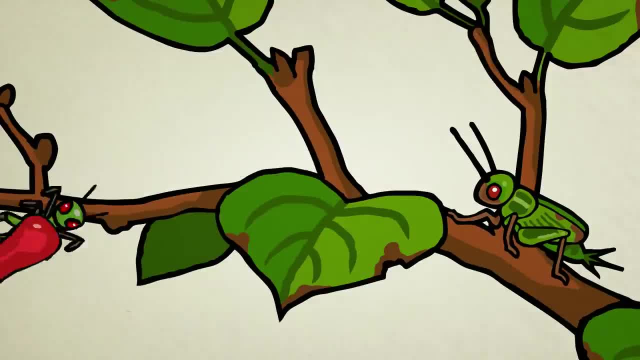 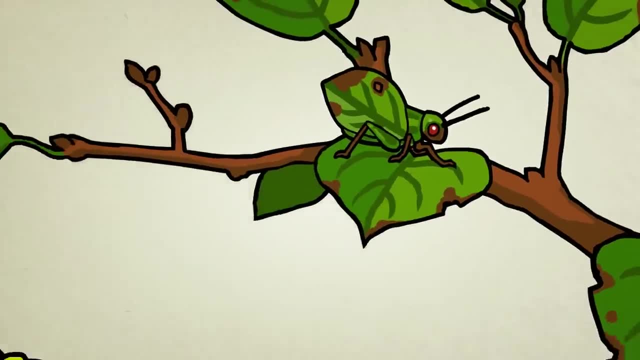 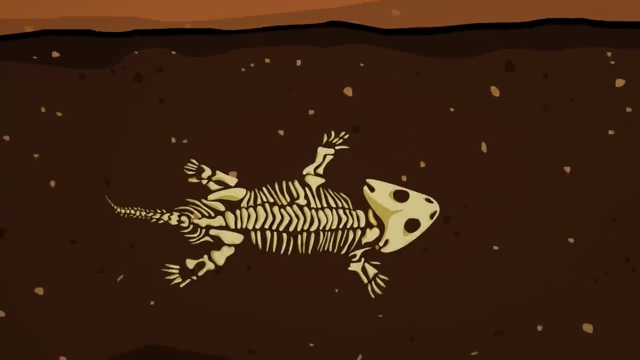 pass those traits on to their children Over multiple generations. positive traits build up, allowing relatively simple life forms to evolve into complex life forms and even split into multiple different species. A careful look at the fossil record overwhelmingly confirms Darwin's theory: Life forms get. 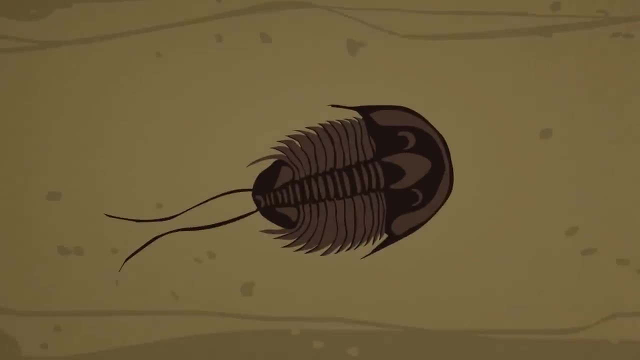 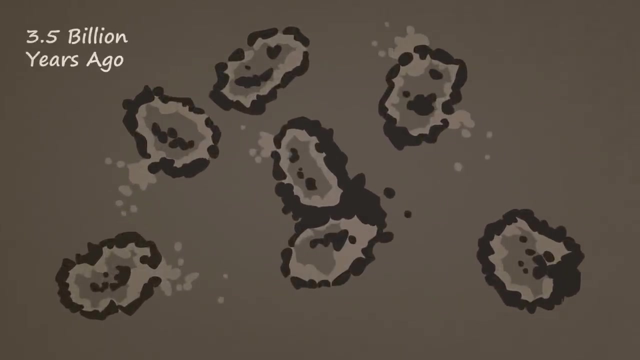 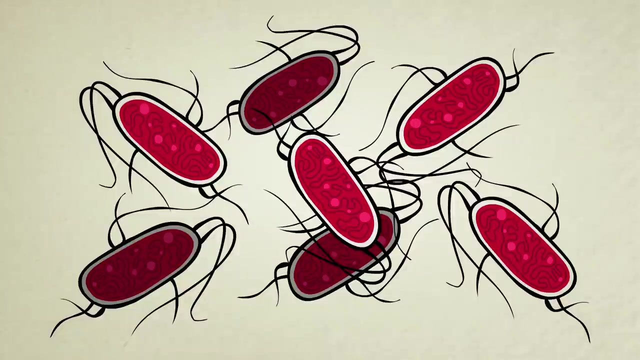 simpler and simpler as we go back in time. The record suggests that all life on Earth emerged from primitive cellular colonies, which first appeared roughly three and a half billion years ago. But how did those first reproducing creatures come about? Even the simplest bacteria alive today are far too complex to have popped into existence. 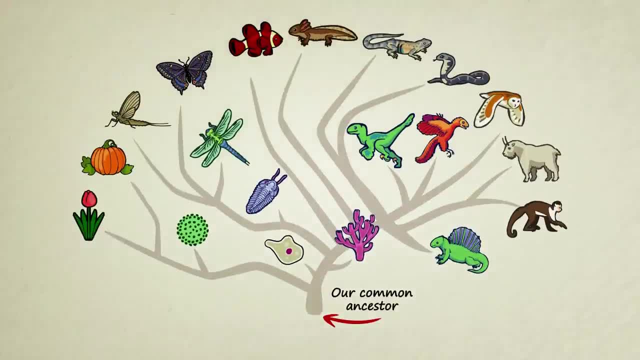 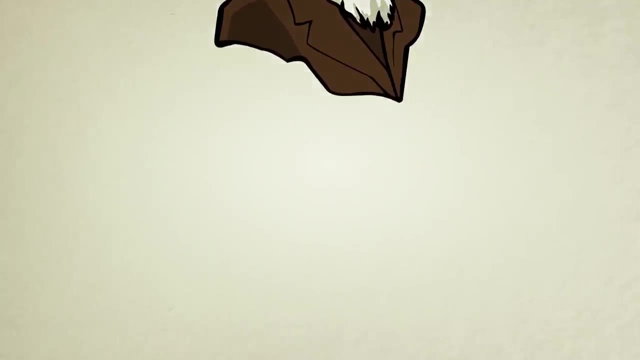 in a single step. Furthermore, the first reproducing creature could not have developed through biological evolution, because biological evolution requires reproduction in order to work. The origin of life needs its own explanation. The most promising idea right now, the one which is consistently leading scientists to new discoveries, is the idea that life emerged. 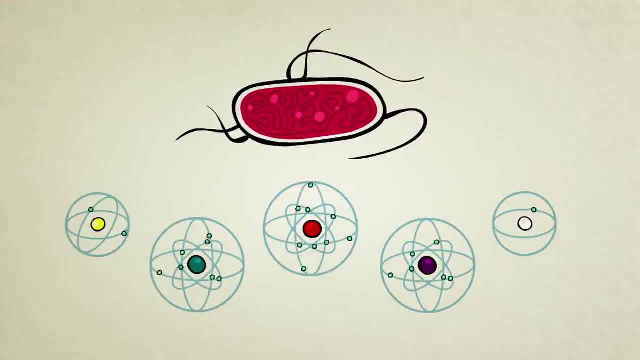 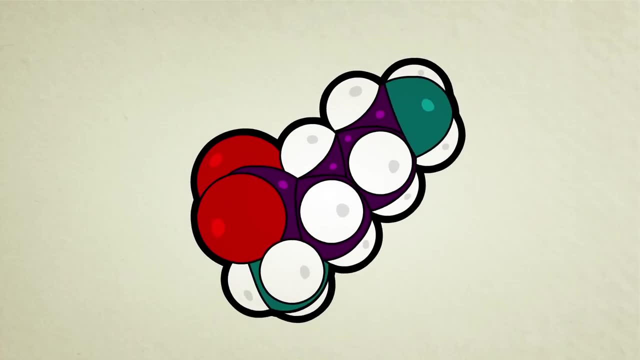 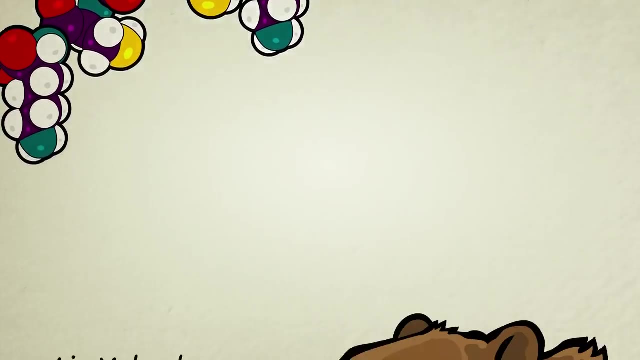 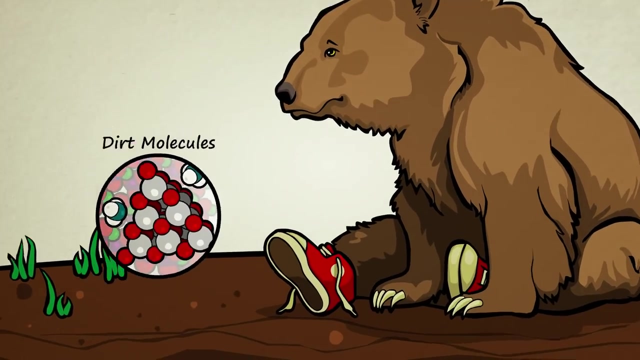 from chemistry. Chemistry is the study of matter, particularly how atoms interact and combine to form molecules, and how those molecules interact and combine to form larger systems and structures. Everything is made of chemicals: The air we breathe, the ground we walk on, the shoes. 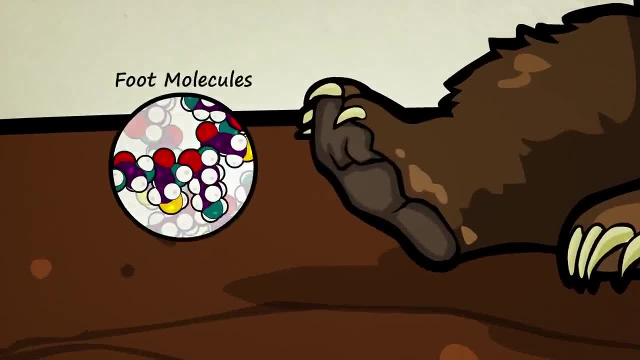 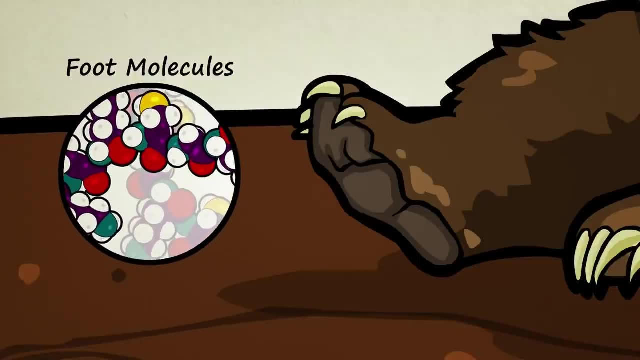 on our feet, even the feet inside our shoes. That said, the chemistry of life is not just about our natural environment and the things we learn about it, but it is about the natural world we meet in life as well. First, the chemistry of life is organized into metabolic pathways. If you look at the 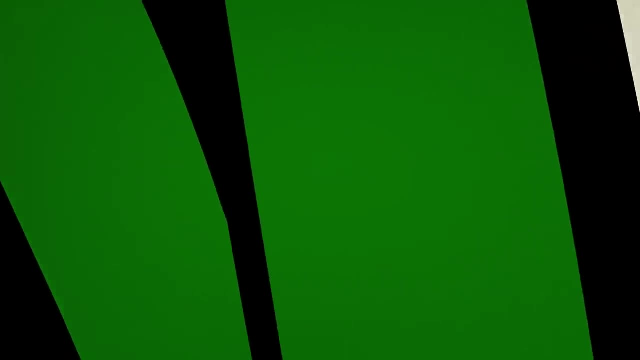 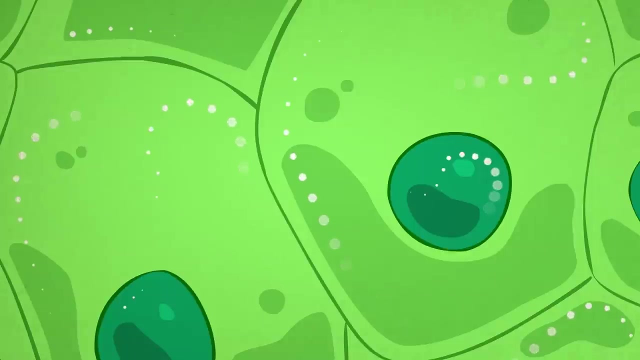 cells of any living thing, even a plant which you wouldn't normally think of as being very lively, you discover a world of activity. Chemical reactions occur in continuously orderly paths, each reaction sparking the next. Scientists call these strange reactions metabolic pathways. 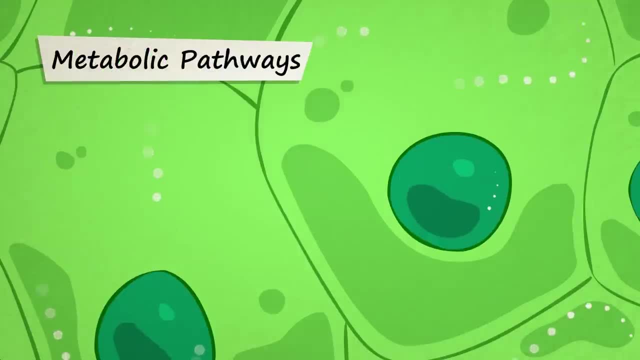 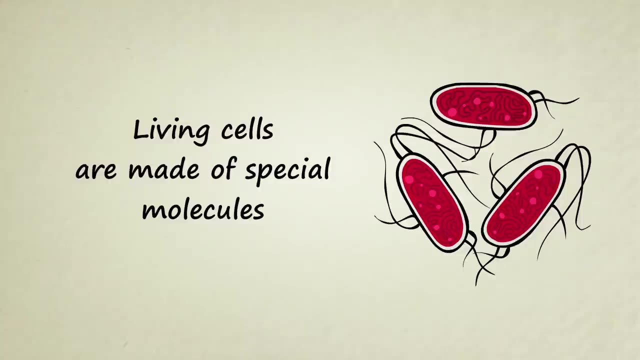 Once we discover any living thing, we can begin to think of it as the world of activities. That's what makes the world of activities so fascinating to me, and so is the world pathways. The second oddity of life's chemistry is that living cells are made of special molecules. 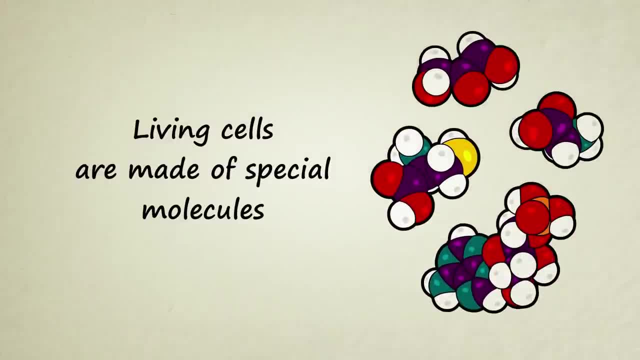 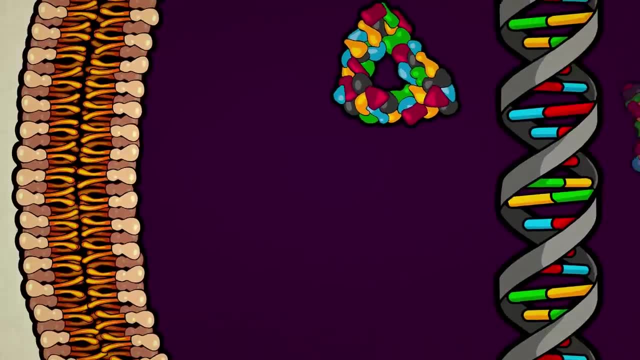 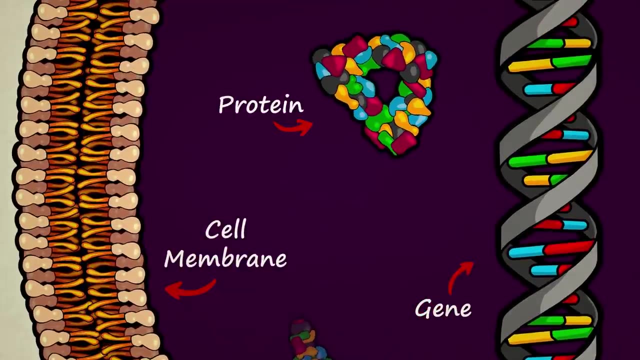 Building blocks like amino acids and sugars, which we once thought could not be found outside of life. These building blocks combine to form highly complex and orderly structures like genes, proteins and cell membranes. In the past, scientists had no idea what powered the strange activities of life and produced 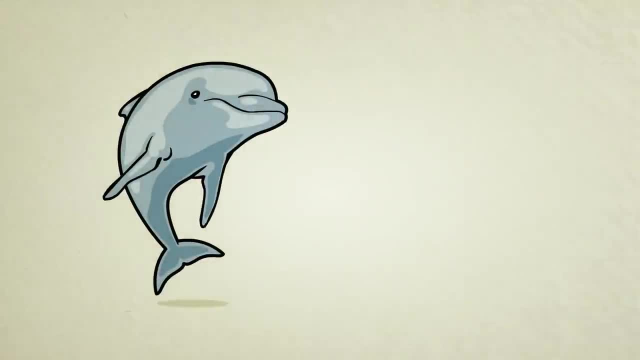 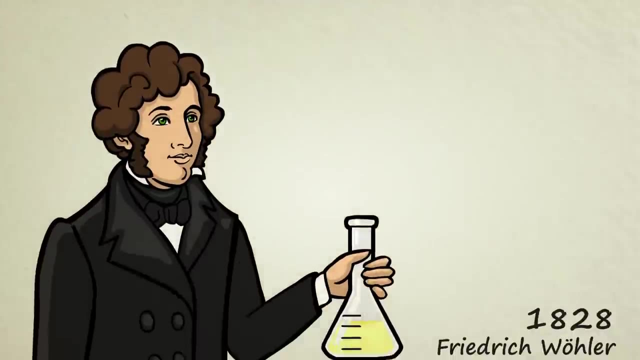 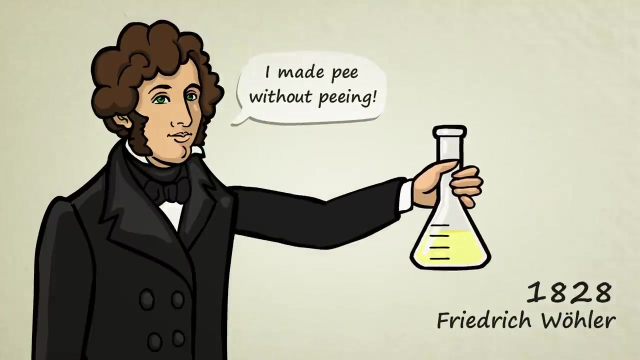 its unique chemicals, They concluded that life must be fueled by a mysterious energy they called the vital force. In 1828, a chemist by the name of Frederick Wuhler accidentally produced urea in his lab. Urea is one of the main components of urine, one of many chemicals that the scientists 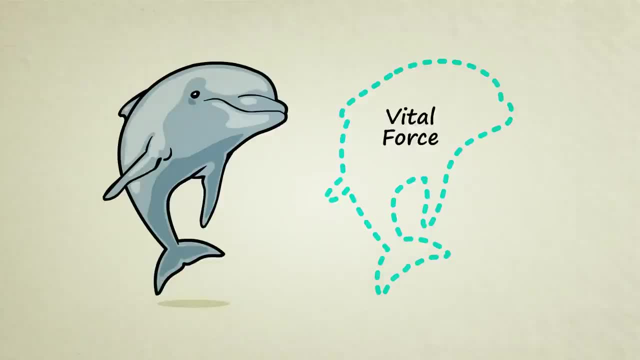 of his time, thought could only be produced by the vital force acting inside of a living creature. The artificial production of urea suggested that life must be fueled by a mysterious energy. they called the vital force. The artificial production of urea suggested that life must be fueled by a mysterious energy. 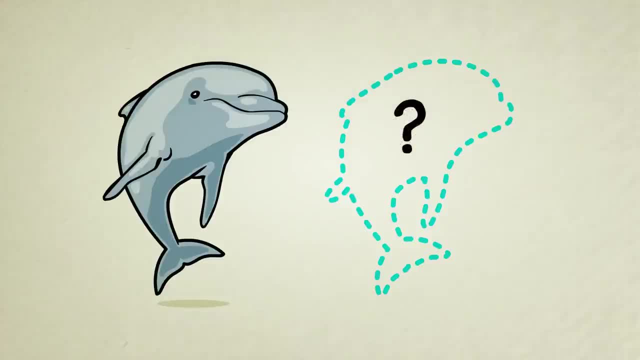 they called the vital force. The artificial production of urea suggested that life must be fueled by a mysterious energy. they called the vital force. The artificial production of urea suggested that life might not be powered by a mysterious force, but instead is powered by normal chemical reactions which could be studied and understood. 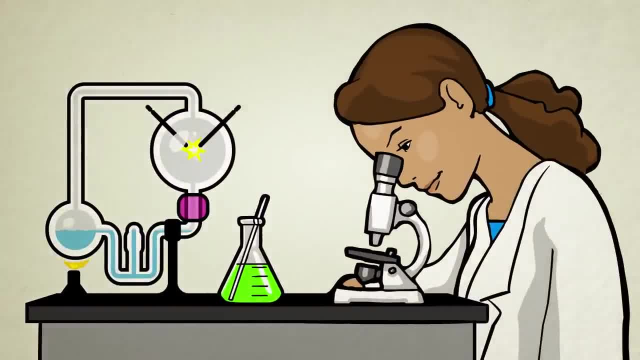 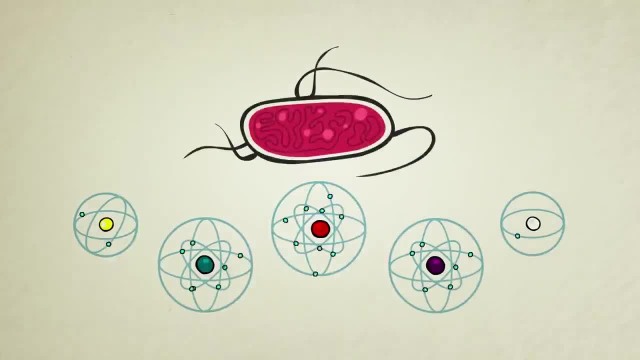 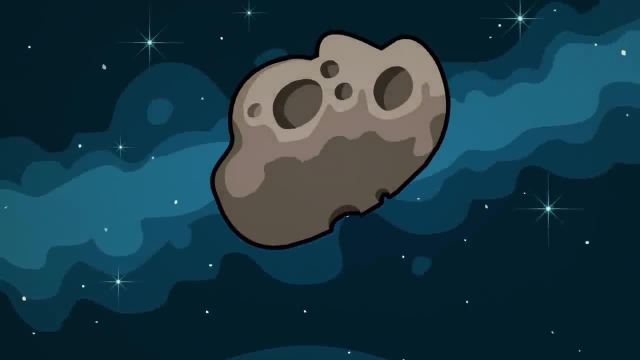 Since that time, numerous molecules and cellular activities have been recreated in the lab, clearly demonstrating that life is powered by normal chemical reactions and suggesting that life may have emerged from non-living. chemistry Researchers have recently discovered that many of the building blocks of life amino 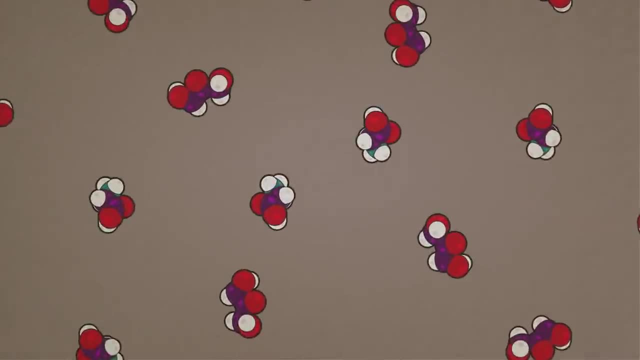 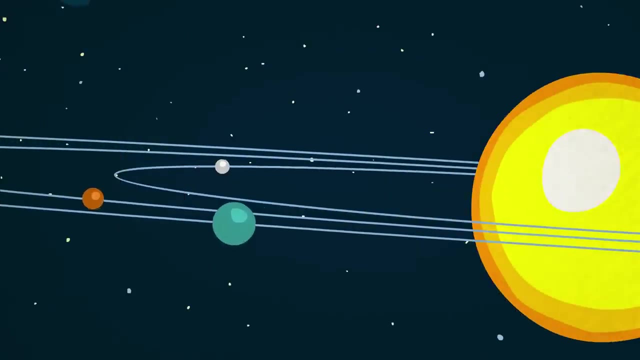 acids and sugars exist inside of life. These blocks are made of meteorites, rocks which have fallen to the earth from outer space. This tells us that these special molecules are being produced spontaneously all throughout our solar system and may have been common on the ancient earth. 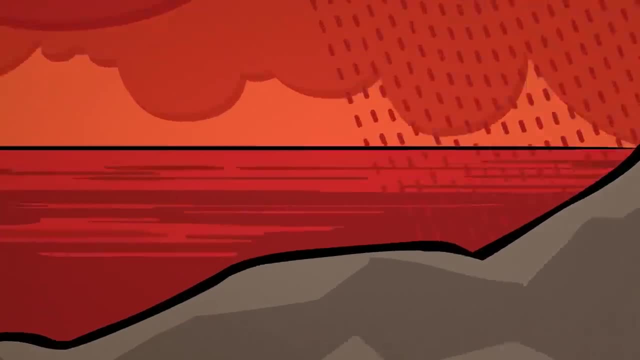 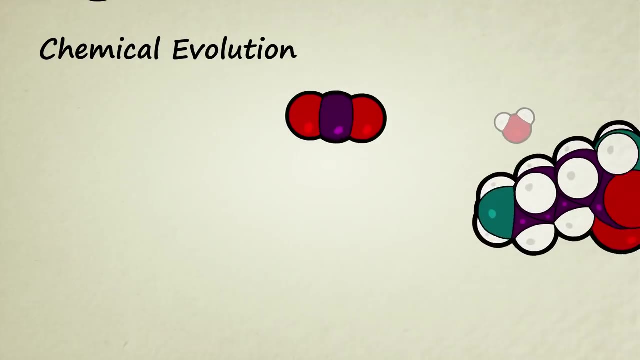 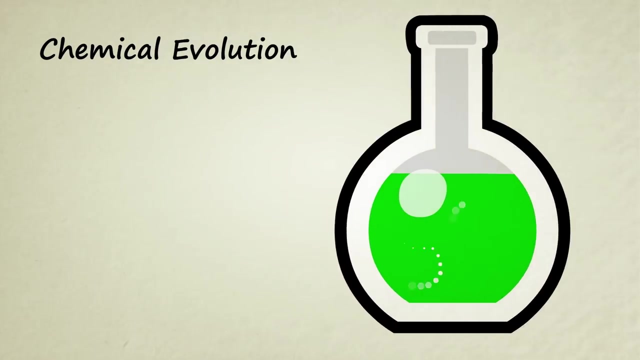 We've also discovered a process now referred to as chemical evolution. When simple molecules are left alone with an energy source, they interact with one another, often forming larger, more complex molecules. as time goes on, Records in the lab have shown that chains of chemical reactions can develop some of 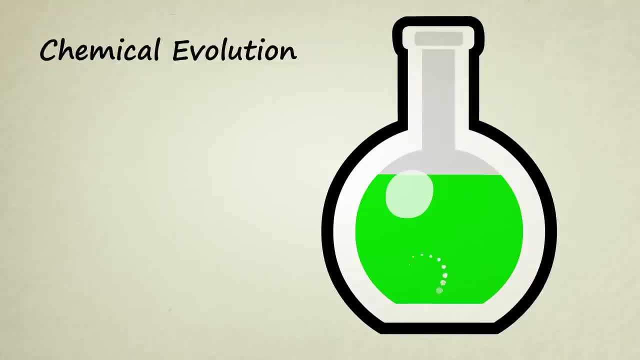 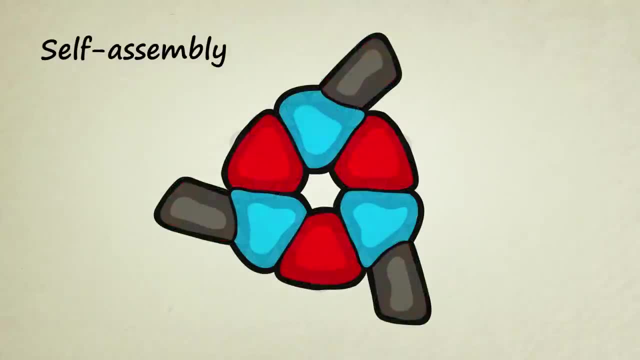 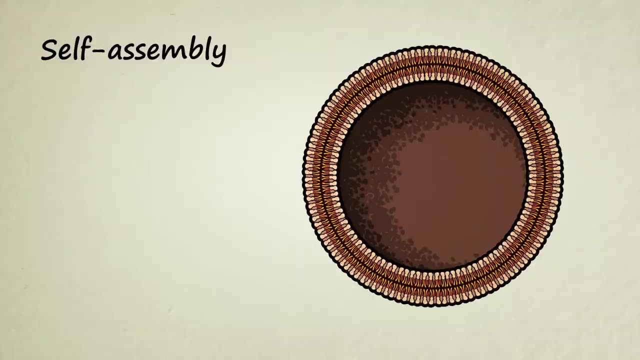 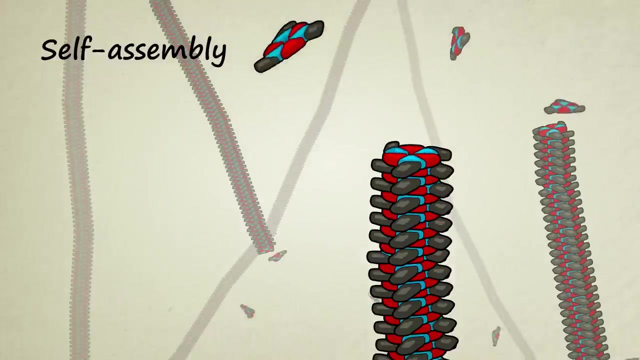 which resemble the metabolic pathways of life. Surprisingly, we've also found that certain molecules have the remarkable ability to self-assemble into complex, orderly structures. Some self-assemble into hollow spheres almost identical to the membranes of modern living cells. others self-assemble into long columns remarkably similar to the strands of DNA found. 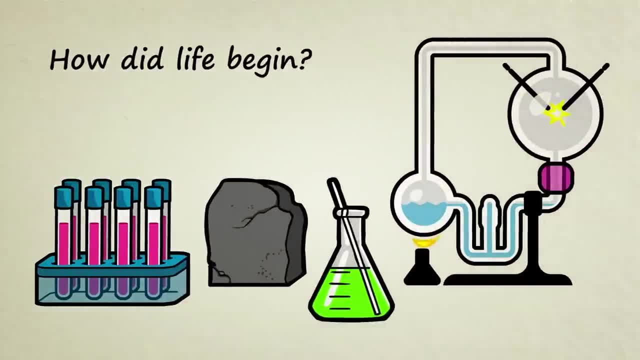 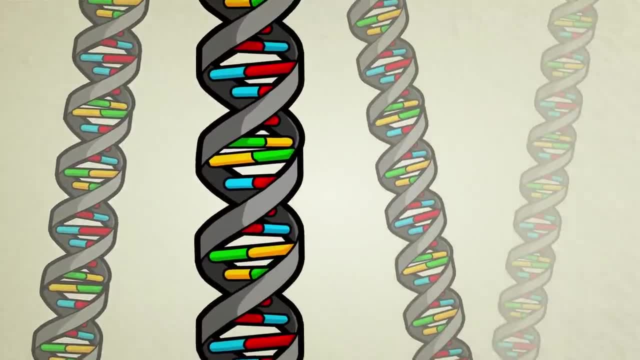 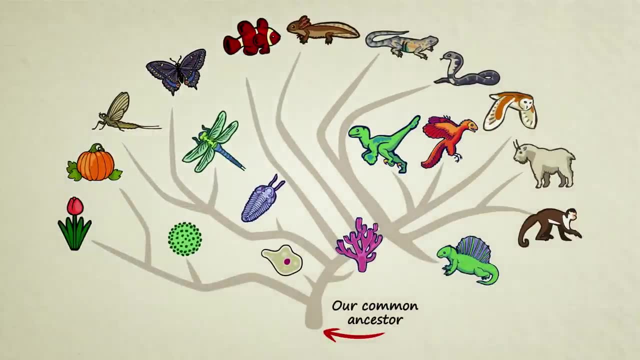 in life. Scientists still have many questions to answer about life's origins. How did different types of molecules first start working together, eventually producing the genetic code? What were the original reproducing creatures actually like? Were they similar to the cells we have today, or were they something much simpler? 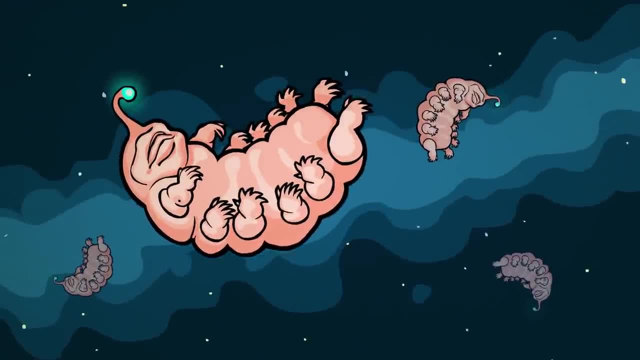 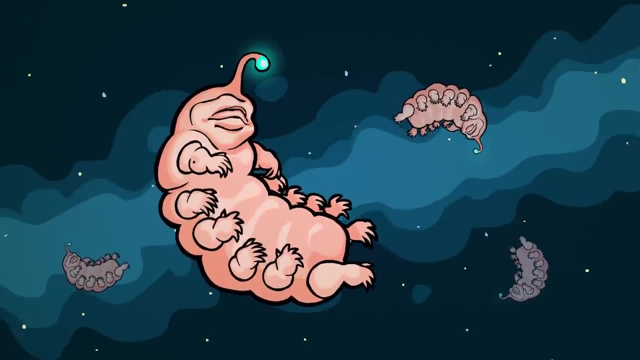 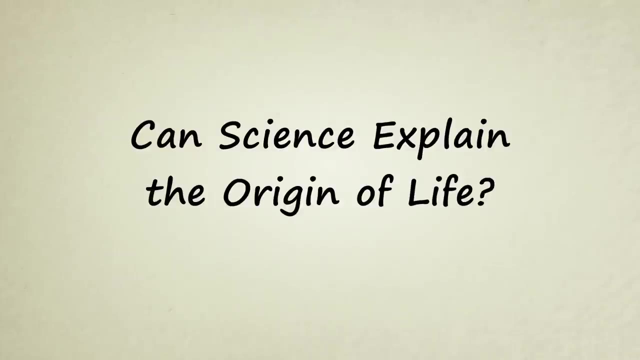 And finally, possibly the most interesting question of all: how likely is it that life has formed or is forming in other regions of our galaxy? So back to the original question: can science explain the origin of life? Science has not explained the origin of life in full detail, but researchers are building. 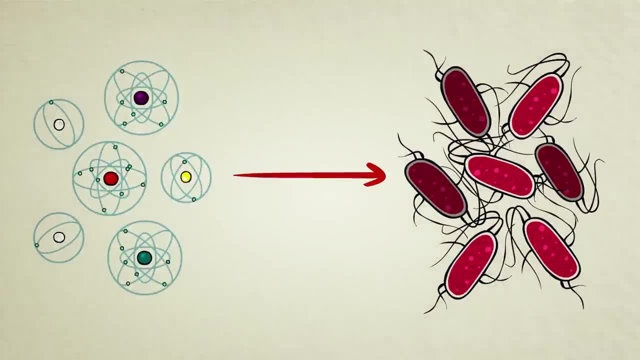 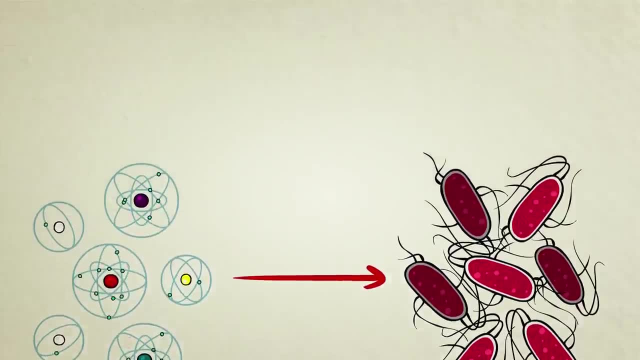 a theory intended to one day describe, start to finish, how basic chemistry can give rise to living cells. I'm John Perry, and that's the origin of life as we understand it, And as we understand it so far, Stated Clearly. 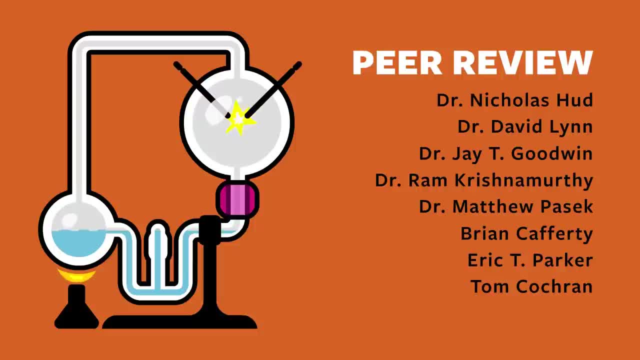 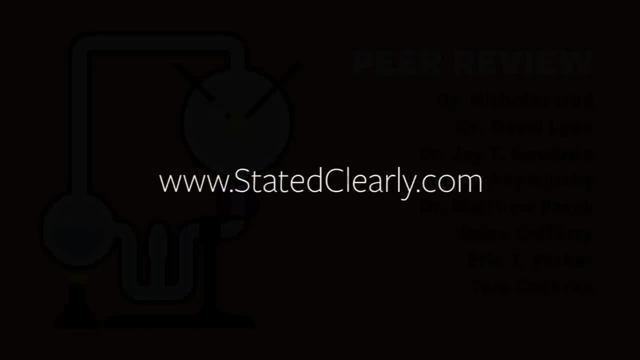 Stated Clearly is a non-profit organization funded by viewers like you. If you'd like to help us fund future projects, visit us at statedclearlycom and click contribute to learn more. Until next time, stay curious.